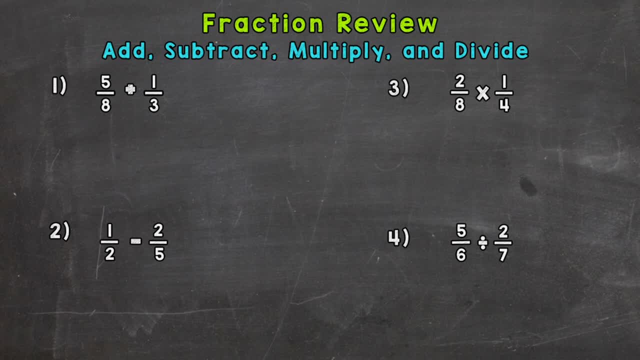 least common multiple is, And the least common multiple for 8 and 3 is 24.. So I'm going to rewrite these fractions below with a denominator of 24.. So what we need to do now is rename them using equivalent fractions so they both have a denominator of 24.. So I know 8 times 3 gives me 24.. So, in order. 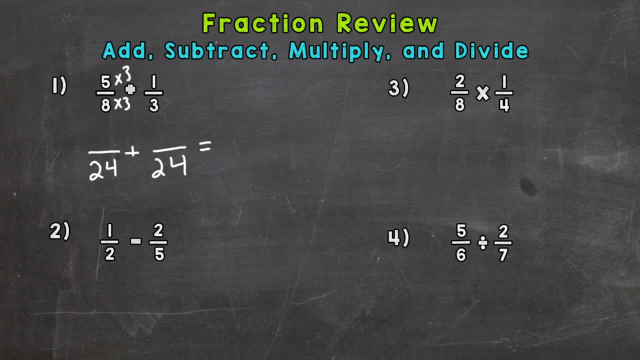 to do that, I need to do the same thing to the top. So 5 times 3 is 15.. So 5 eighths is equivalent to 15 twenty-fourths. Now for 1 third, 3 times 8 gives me that 24.. So I need to do the same thing. 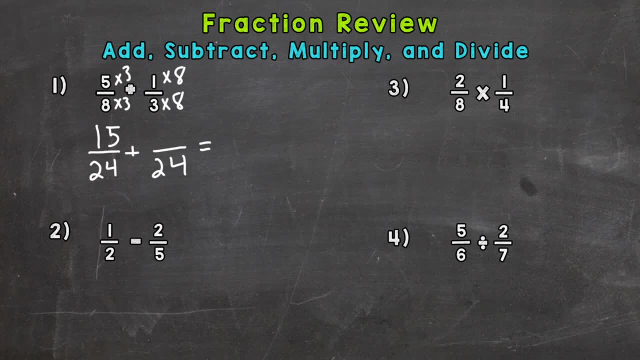 to the top: 1 times 8 is 8.. So now that I have the renamed fractions with a denominator of 24, I can add my numerators: 15 plus 8 is 23.. And you always keep your denominator the same. 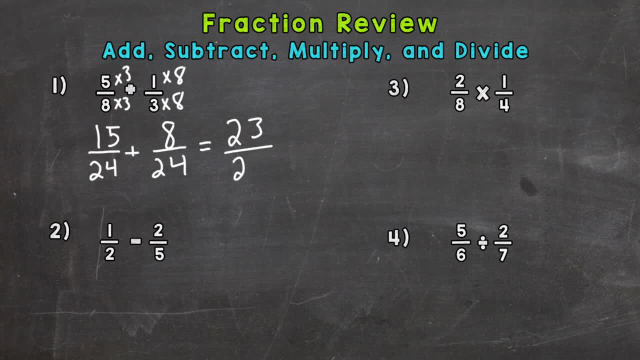 whatever that common denominator is, which it is 24.. Then check to see if your answer can be simplified, If there's a common factor that I can divide both my numerator and denominator by. Well, the only common factor is 1 here. so we are in simplest form, So I'm going to do the same thing. 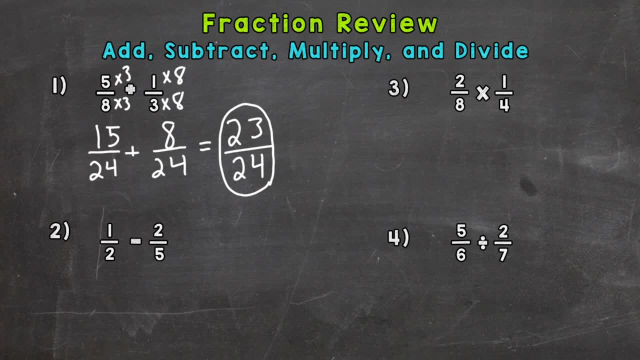 in the simplest form, Our answer is 23 twenty-fourths. So number 2, on to subtraction, And subtraction is the same exact thing as addition. You just subtract instead of add. So we have 1 half minus 2 fifths. We obviously don't have a common denominator there, so we are not able to subtract. 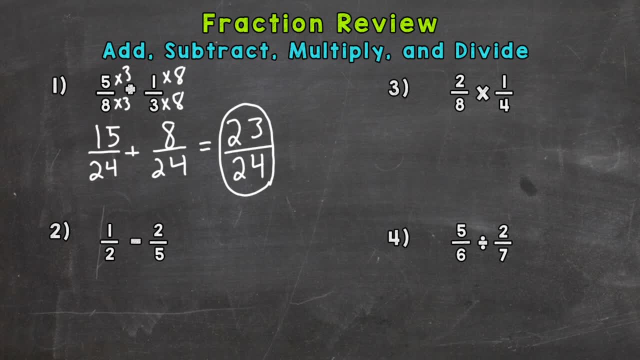 right off the bat. So we need to find a common denominator which, again, is going to be your least common denominator. So we need to find a common denominator which, again, is going to be your least common denominator. So we need to find a common denominator which, again, is going to be your least. 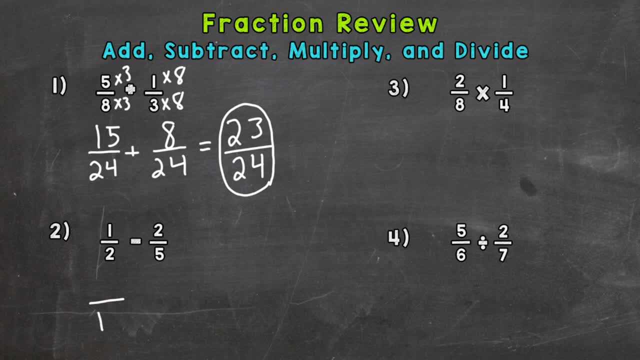 common denominator. So we need to find a common denominator. So 2 and 5 are least common. so 2 and 5 are least common will be 10.. I know 2 times 5 is 10, 1 times 5 will be 5.. So 1 half is equivalent to five tenths. I need to do the same thing to the top. So I need to do the same thing to the top. So I need to do the same thing to the bottom. So now that I have the renamed fractions with a denominator of 24, 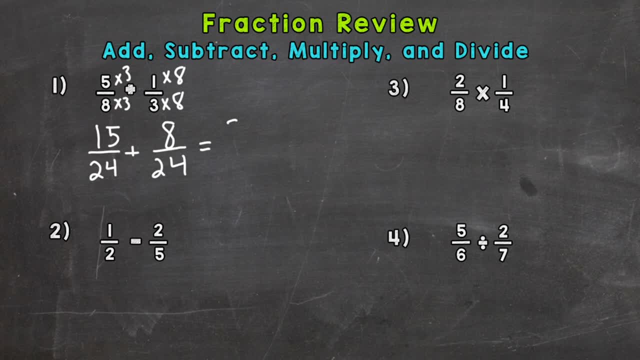 I can add my numerators. 15 plus 8 is 23. And you always keep your denominator the same, whatever that common denominator is, which it is 24. Then check to see if your answer can be simplified. If there's a common factor that I can divide both my numerator and denominator by. 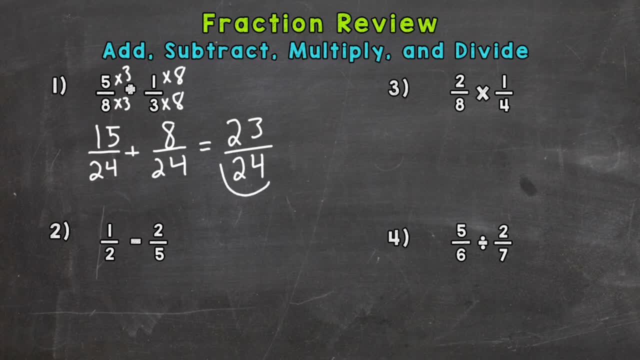 Well, the only common factor is 1 here. So we are in simplest form. So the answer is 23 twenty-fourths. So number 2, on to subtraction. And subtraction is the same exact thing as addition. 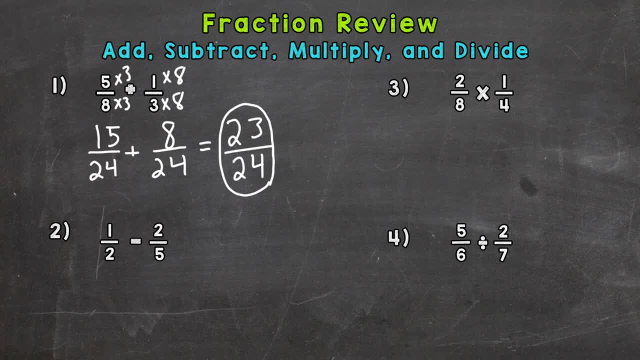 You just subtract instead of add. So we have 1 half minus 2 fifths. We obviously don't have a common denominator there. So we are not able to subtract right off the bat. So we need to find a common denominator, which again is going to be your least common multiple. 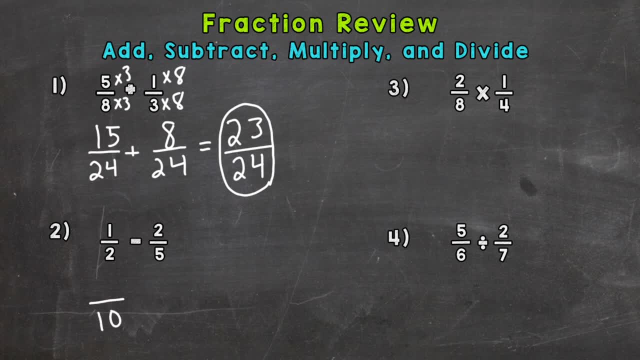 So 2 and 5, our least common multiple, is going to be 10. I know 2 times 5 is 10. 1 times 5 is 5. So 1 half is equivalent to 5 tenths. Now on to two fifths here. 5 times 2 gives me that denominator of 10. So 2 times 2 gives me 4. 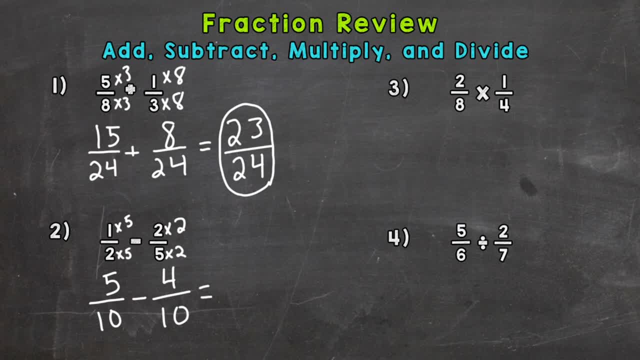 Now I'm ready to subtract. 5 minus 4 is 1 and we keep our denominator of 10 the same. So 1 tenth is our answer. Now you always look to simplify just like number 1 there 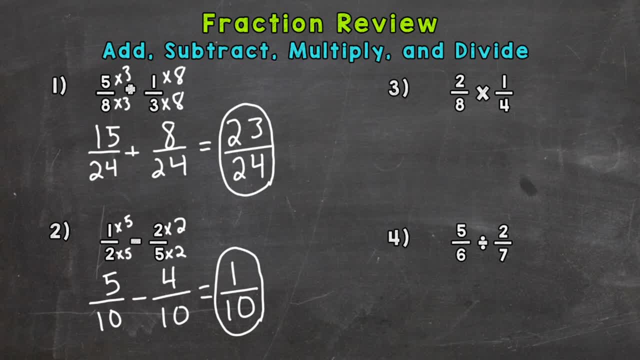 but our only common factor between 1 and 10 is 1 so we are in simplest form. 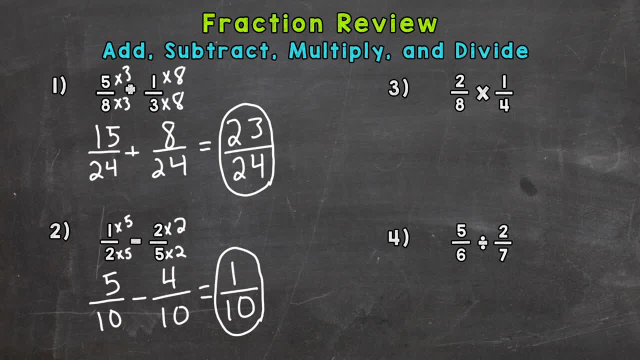 Number 3, multiplying fractions. So with multiplying fractions we do not need a common denominator. You actually just multiply straight across. So you go numerator times numerator and denominator times denominator. So 2 times 1 is 2 and 8 times 4 is 32. So that's our answer. 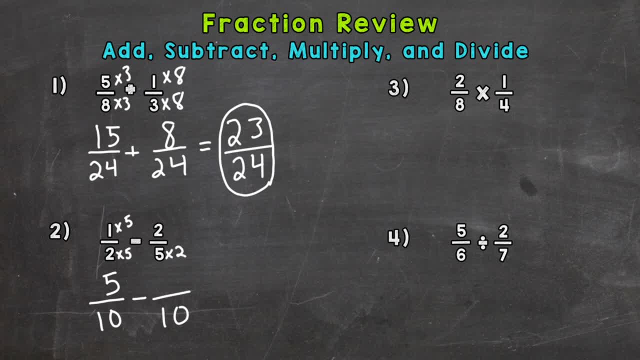 so 1 half is equivalent to five tenths. Now on to two fifths here. 5 here, 5 times 2 gives me that denominator of 10.. So 2 times 2 gives me that denominator of 10.. So 2 times 2 gives me 4.. of 2 times 3 gives me 4.. 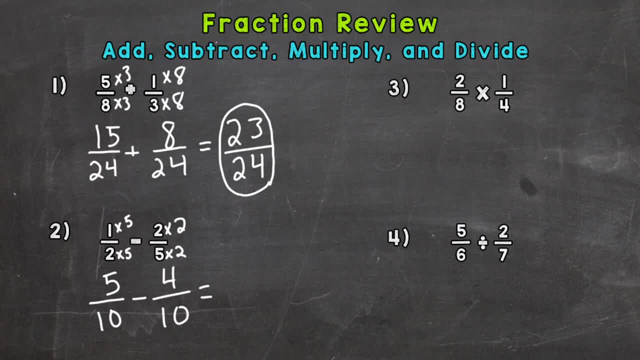 4.. Now I'm ready to subtract: 5 minus 4 is 1, and we keep our denominator of 10 the same, So 1 tenth is our answer. Now you always look to simplify, just like number 1 there. 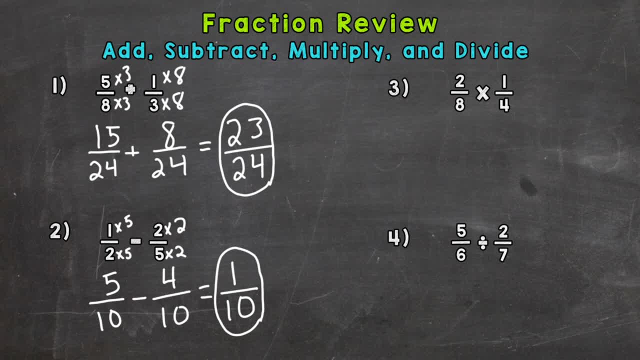 but our only common factor between 1 and 10 is 1, so we are, in simplest form, 6.. Number 3, multiplying fractions. So with multiplying fractions we do not need a common denominator. You actually just multiply straight across. So you go: numerator times numerator and denominator times denominator. 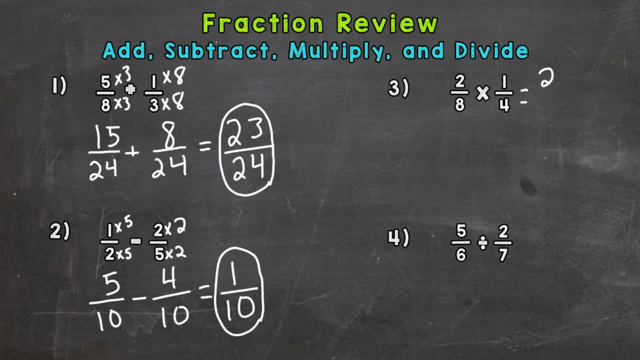 So 2 times 1 is 2, and 8 times 4 is 32.. So that's our answer. Now, this fraction can't be multiplied, It can be simplified. There's a common factor between 2 and 32, so we can break this fraction down. 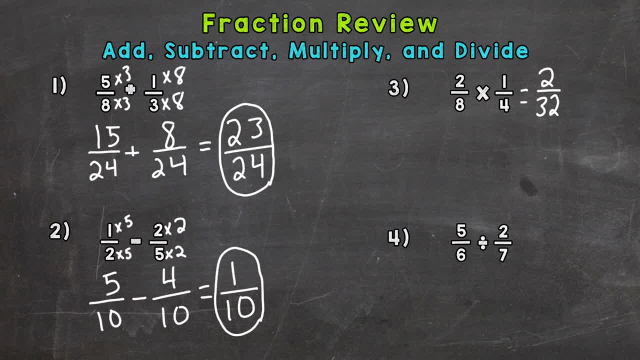 The common factor between 2 and 32 is 2.. So I can divide both of them by 2, and I will get the equivalent fraction, which is our simplest form of 2 over 32, which 2 divided by 2 is 1, and 32 divided by 2 is 16.. 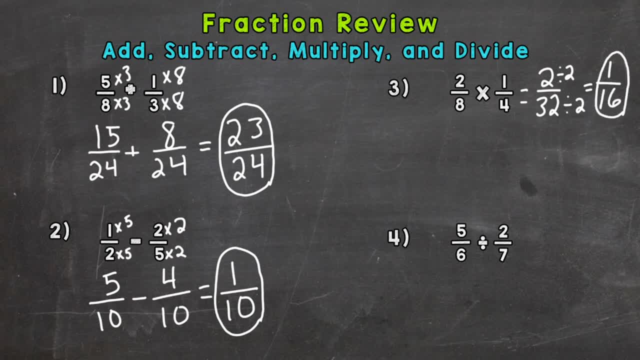 So our simplest form. So the answer here is: 1 sixteenth Number 4, 5 sixths divided by 2 sevenths. Now for dividing fractions. we keep switch and flip, So whatever our first fraction is, we always keep it. 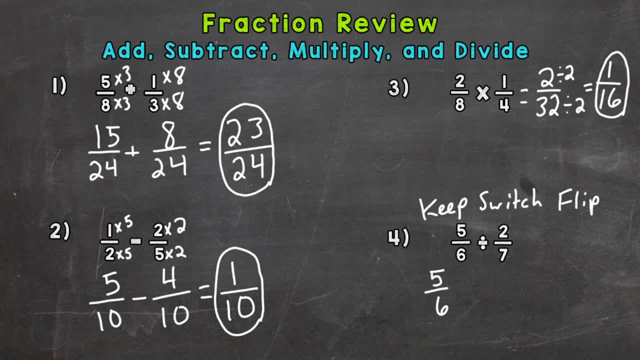 We switch the division sign And we flip the second fraction. So the 7 is going to be our numerator and the 2 is going to be the denominator. Keep, switch, flip. 5 times 7 is 35.. And 6 times 2 is 12.. 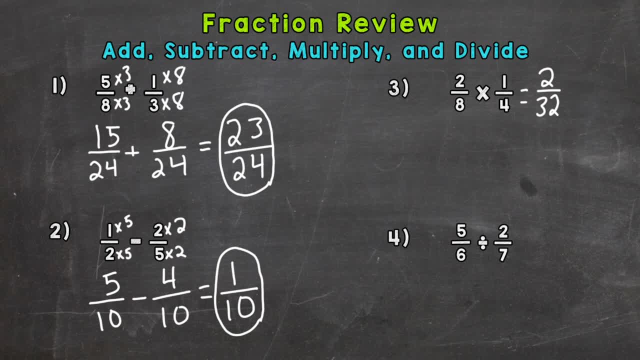 Now this fraction can't be multiplied. It can be simplified. There's a common factor between 2 and 32 so we can break this fraction down. The common factor between 2 and 32 is 2. So I can divide both of them by 2 and I will get the equivalent fraction which is our simplest form of 2 over 32 which 2 divided by 2 is 1 and 32 divided by 2 is 16. So our simplest form. So the answer here is 1 sixteenth. 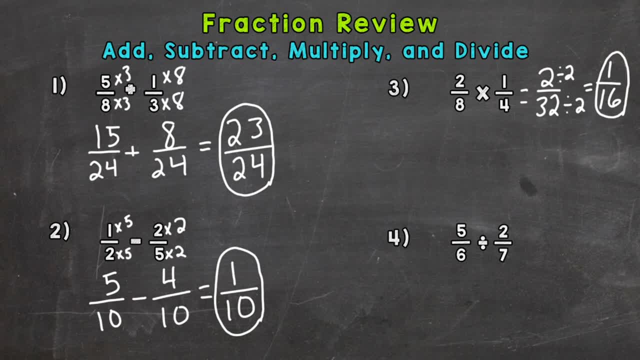 Number 4, 5 sixths divided by 2 sevenths. Now for dividing fractions we keep, switch, and flip. 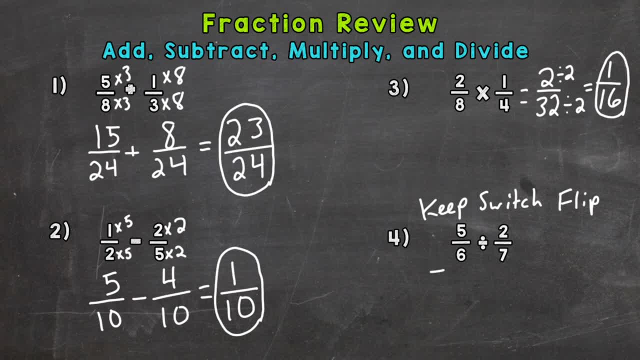 So whatever our first fraction is we always keep it. We switch the division sign. To multiplication. And we flip the second fraction. So the 7 is going to be our numerator and the 2 is going to be the denominator. Keep, switch, flip. 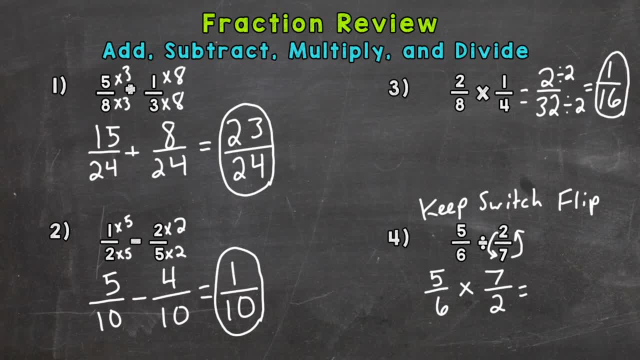 5 times 7 is 35. And 6 times 2 is 12. This gives us an improper fraction and we don't want to leave it like that. 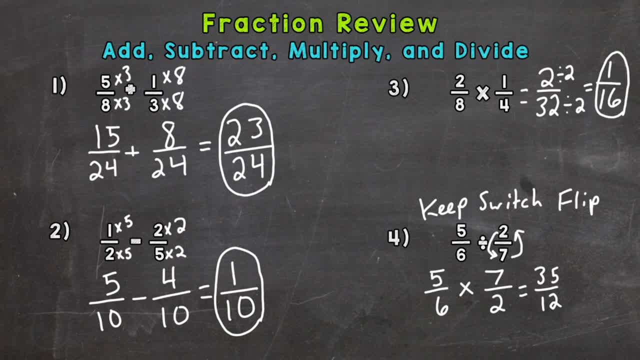 We want to convert this to a mixed number. So essentially it's 35 divided by 12. How many whole 12s can we pull out of 35? And that's going to be our whole number. And so if we think about it, if we count up by 12s. 12, 24, 36. So 3 twelves is a little bit too much. So it's only going to be 2 whole 12s which gets us to 24. That means we have 11 left over. 11 left over. 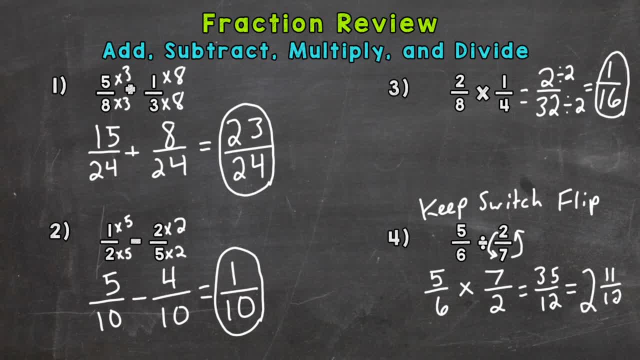 As our remainder. And we keep our denominator of 12 the same. So again I did 35 divided by 12. 2 whole 12s can be pulled out of 35. With 11 left over. 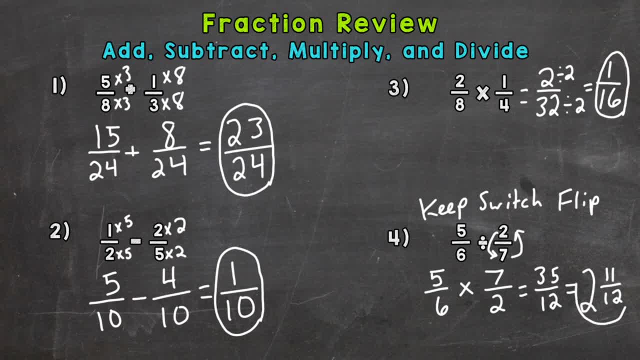 And you keep your denominator of 12 the same. And 11 twelves cannot be simplified. So we are done with number 4.